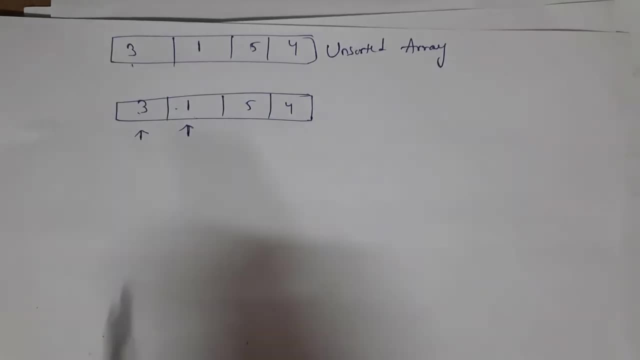 should be 3.. Definition of bubble sort is: we need to swap adjacent elements if they are in wrong order. So adjacent element of 3 is 1.. Now we need to swap this 3 and 1.. After swapping my array. 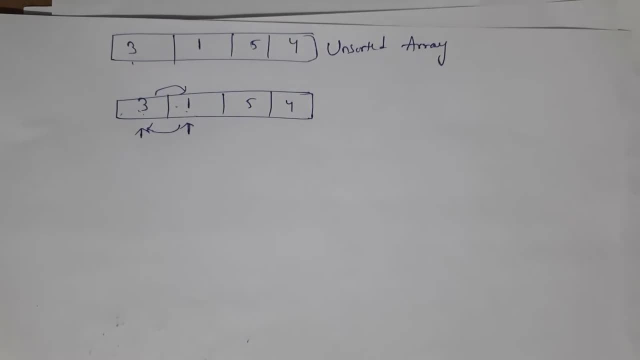 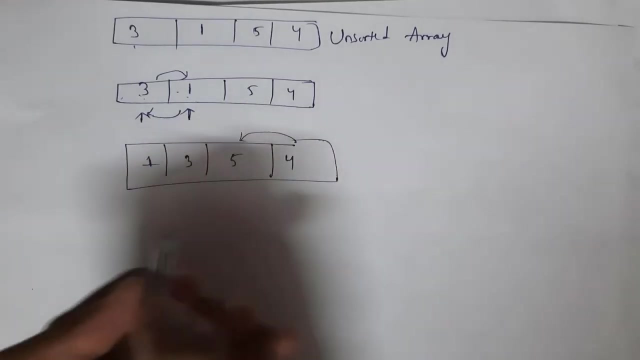 look like this: We need to swap 3 and 1.. So, after performing swapping, my array look like this: 1, 3, 5, 4.. This array is not sorted because 4 must be here and 5 must be here, So again, we need to swap this. 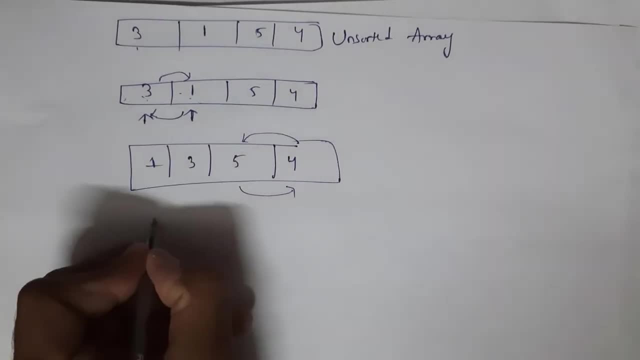 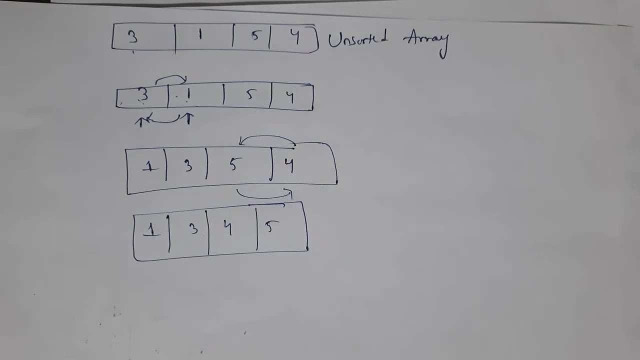 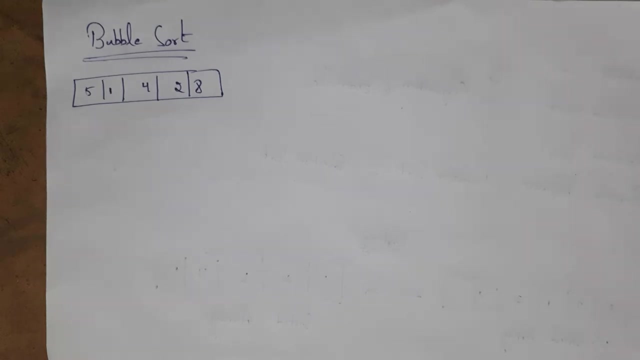 adjacent elements. After performing swapping, my array look like this: 3 swap, 4 and 5.. Now my array is in sorted manner. This is how we sort elements by using bubble sort. This is an unsorted array. Now we need to sort this array by using bubble sort. We should sort from first element and then 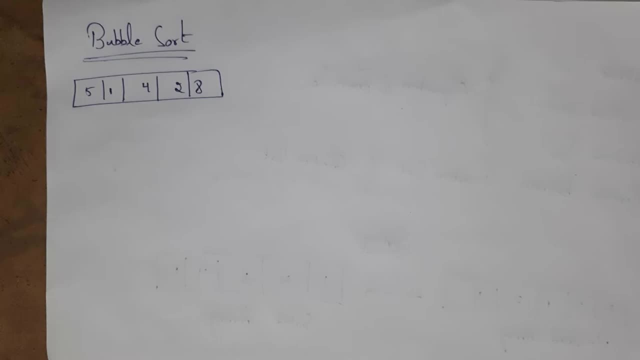 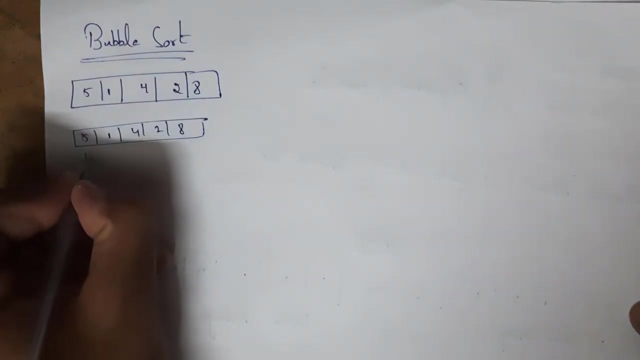 we should keep on checking each and every element, whether these elements are in correct position or same as it is: 5, 1, 4, 2 and 8.. Now place cursor to first position. First element is 5 and next move cursor to next position. Next element is 1.. These both are not in proper order, because one must be. 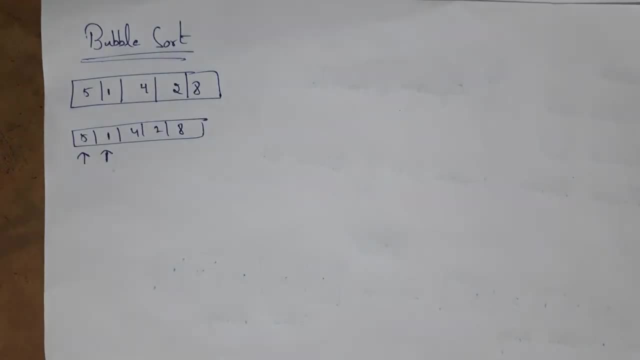 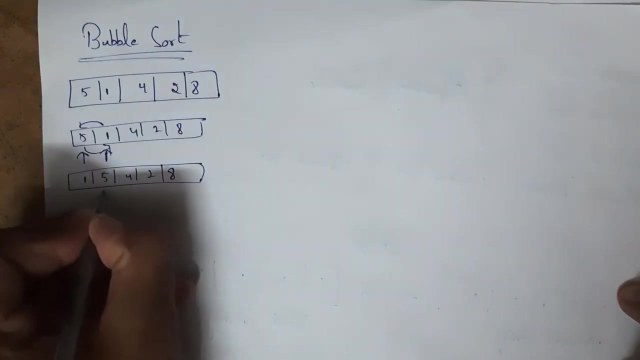 first and after one there should be 5.. So these both are in wrong order, So swap this. adjacent elements. Adjacent element of 5 is 1.. So we will swap this both: 1, 5, 4, 2 and 8.. My cursor is here. 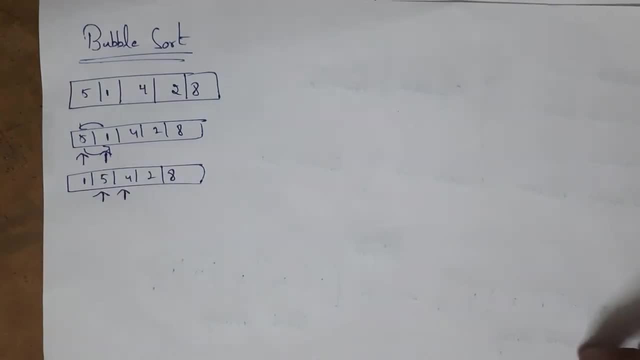 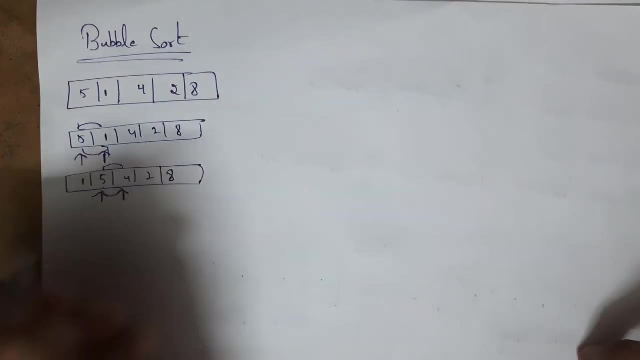 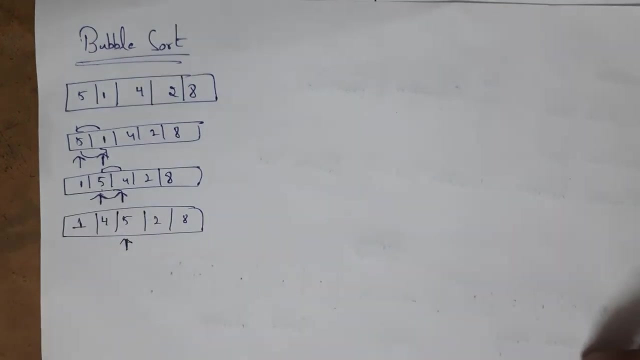 Now move cursor one position forward. So I am placing cursor here. Here is 5 and 4.. Both are in proper order. So again, swap this, both adjacent elements. So after swapping my array look like this: 1, 4, 5, 2, 8.. My cursor is here. Now move cursor one position forward and compare this: both 5 and. 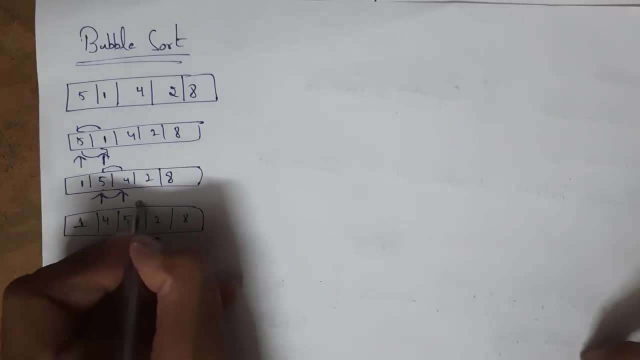 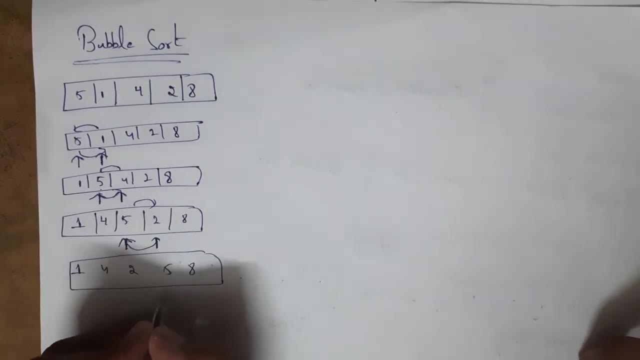 2. 2 should be first and after 2 there should be 5.. So again, swap this 5 and 2.. Swap this adjacent elements. So after swapping my array look like this: 1, 4, 2, 5, 8.. Now my cursor is here. 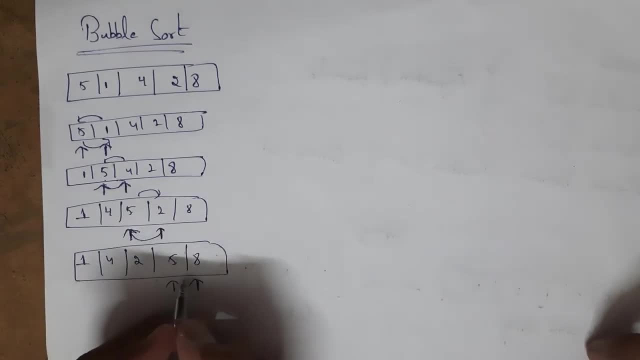 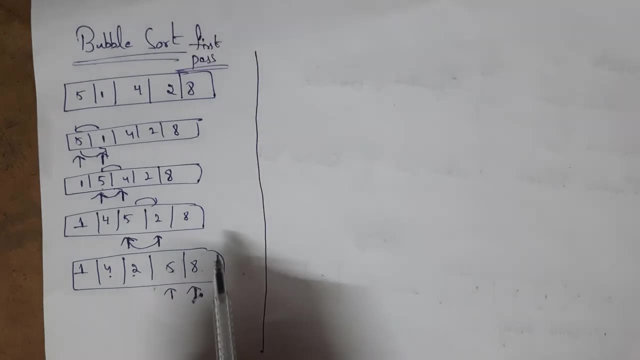 and move cursor to next position. So my cursor reach to last position. Both are in correct order, So there is no need of swapping Here. cursor reach to last position, but elements are not in proper order. That is still. it is unsorted array, So consider it as. 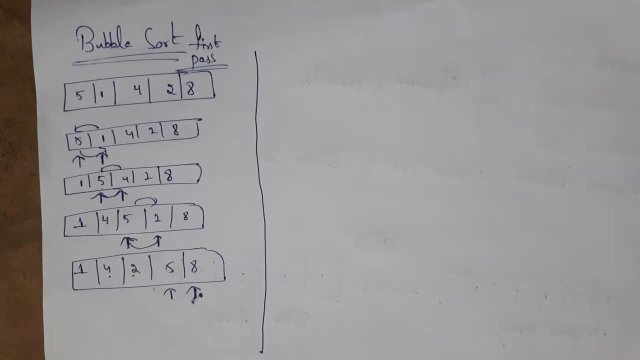 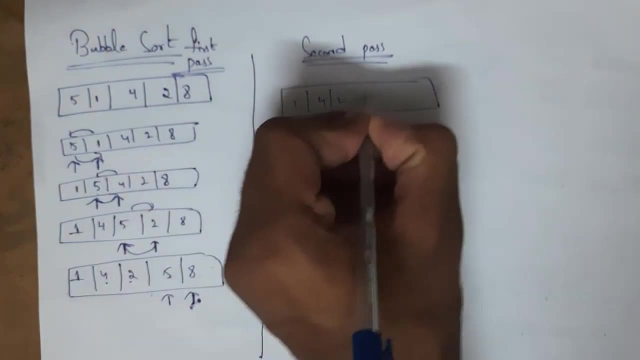 first pass and we need to start second pass. and again, we should keep on sorting the elements. This is second pass. Write this elements here: 1, 4, 2, 5, 8. 1, 4, 2, 5, 8.. Again, we should start sorting. 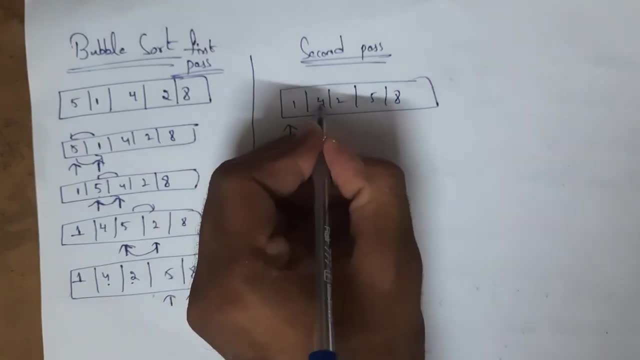 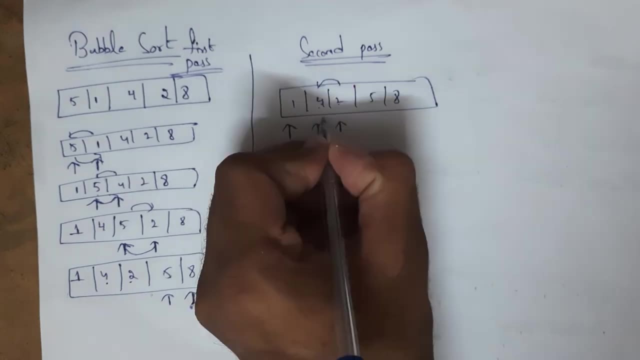 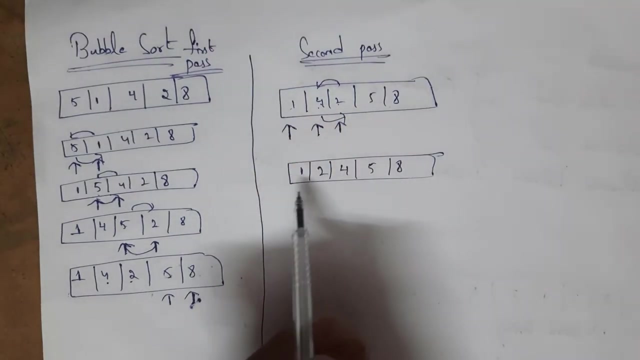 from first. Move cursor to next position 1 and 4.. Both are in correct order, So again move cursor to third position Here. 2 should be here and 4 should be here, So exchange this: both adjacent elements. After sorting my array look like this: 1, 2, 4, 5 and 8.. Now all these elements are in. 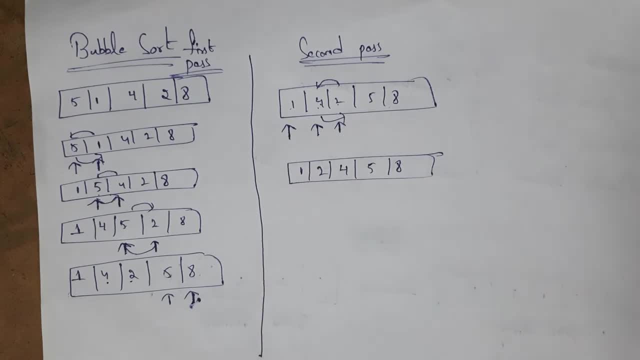 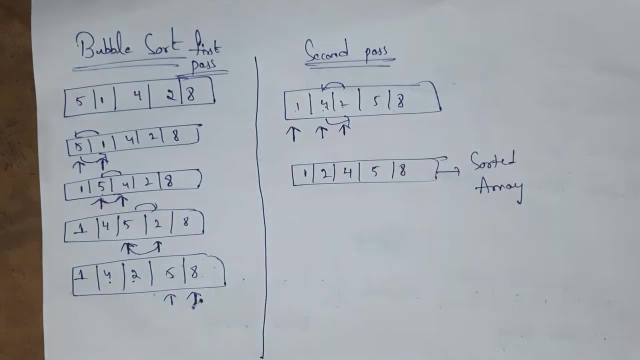 ascending order that is from small to big. So we can stop sorting Now. this is considered as sorted array because all these elements are in proper order: sorted array. This is how we perform sorting by using bubble. sort Guys roughly. I explained, but you need to write this in step. 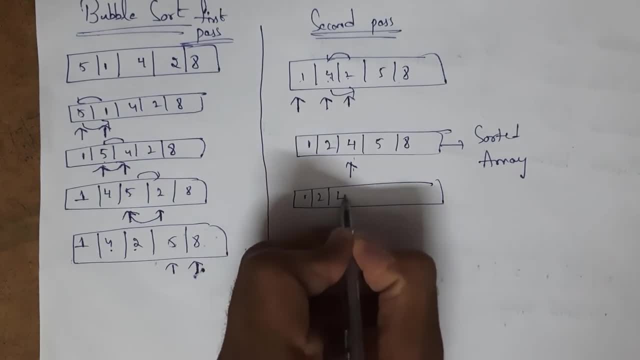 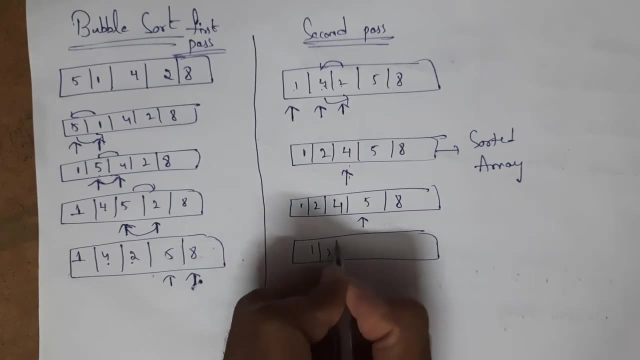 my cursor is here, So you need to perform checking until last element. So again, move cursor here and again take another step. 1, 2, 4, 5, 8. From 8: you need to move cursor here Whenever this cursor is. 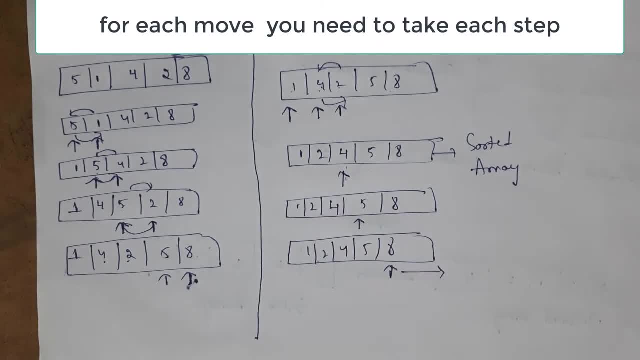 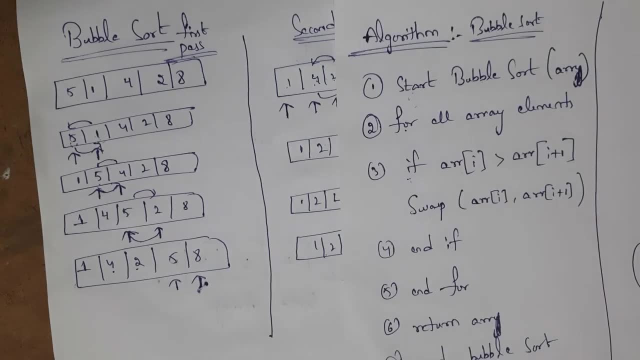 reach to last position, then you need to check these elements, whether these elements are in correct position or not. This is how we perform bubble sort. I will explain. algorithm of bubble sort. This is an algorithm for bubble sort. Step 1 is start bubble sort of array. 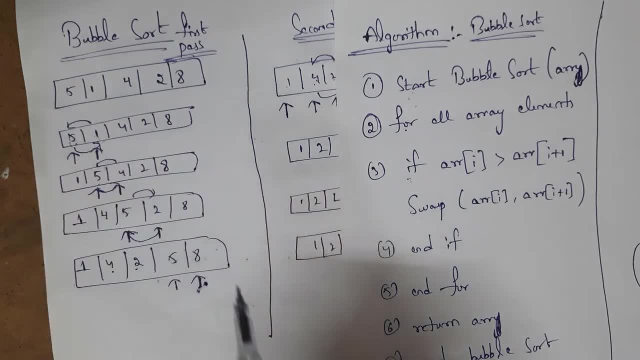 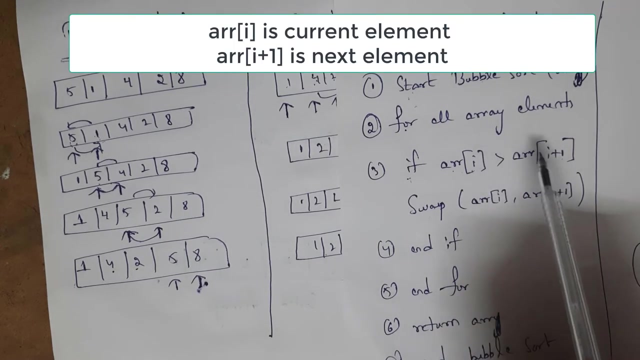 Because we are performing bubble sort on array of elements. So here step 1 is: start bubble sort array and next step is, if array i is greater than array i plus 1, swap array i comma, array i plus 1.. That mean if first element is greater than next element, then we need to swap this, both elements. 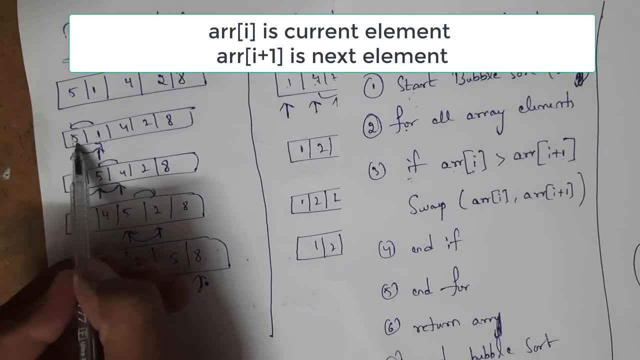 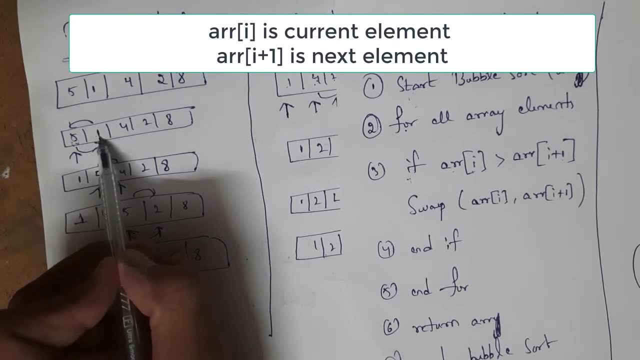 This is meaning of this step. If you consider this example here, first element is 5 and next element is 1.. This 5 is greater than 1, because actually 1 should be first and after 1 there should be 5.. This, both are in. 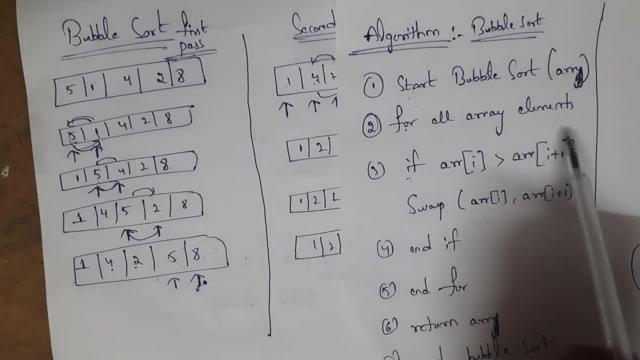 Wrong position, So we need to interchange this. both elements. We need to perform this step for all the elements present in an array. We need to close this if condition, So step 4 is end if and after that we need to close this for loop, So step 5 is end for After that we need: 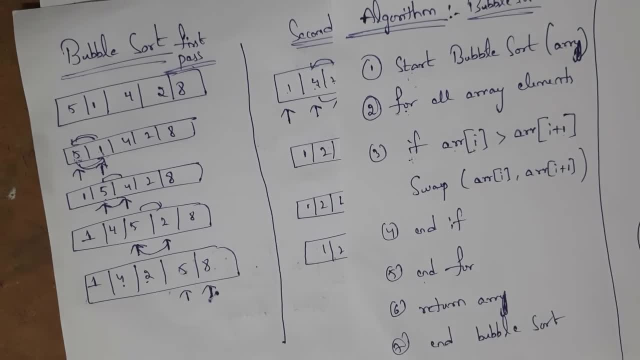 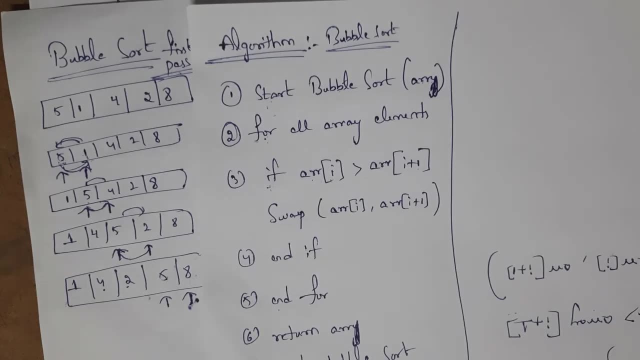 to return array and at last we need to end bubble sort. This is algorithm for bubble sort. You need to remember definition of bubble sort, that is, we swap adjacent elements if they are in wrong position. Next I will explain what is selection sort. This selection sort algorithm sorts an array. 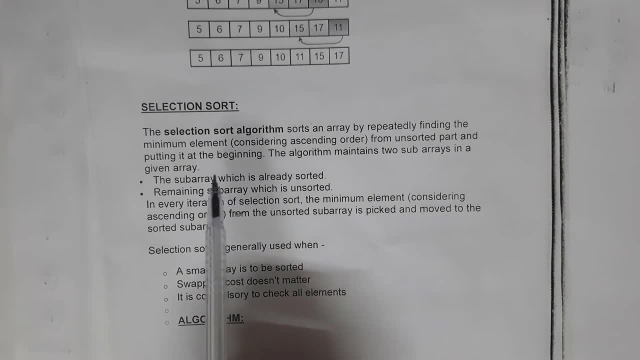 of elements and then selects the selected array. This selection sort maintains two arrays: one is sorted array and one is unsorted array. I will give one example so that you can clearly understand how selection sort will work. This is unsorted array. Now we need to sort this array by using 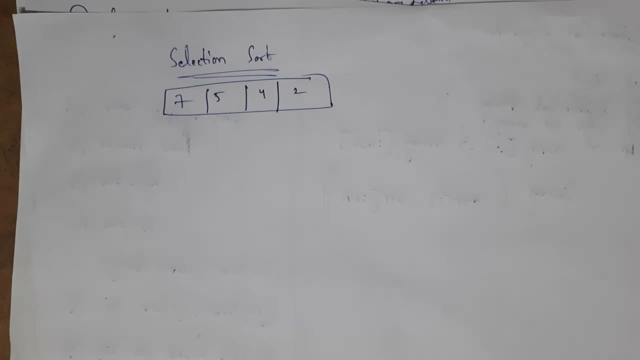 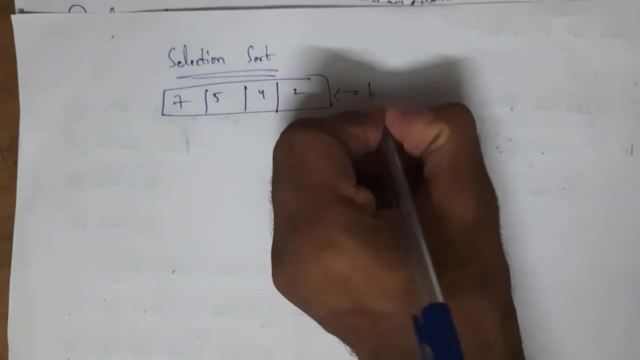 selection sort. Selection sort maintains two arrays: One is sorted array and one is unsorted array. So let us consider this as unsorted array, because this is not in proper order. So consider it as unsorted array. Selection sort will find minimum element. 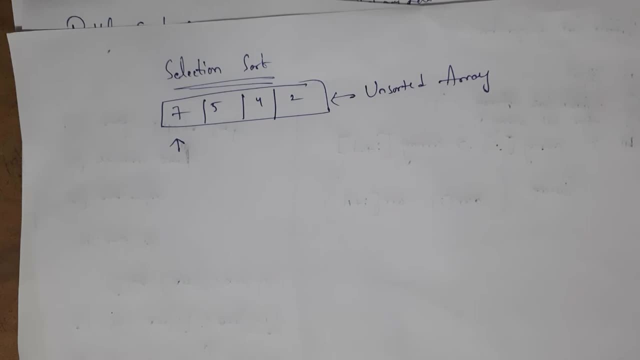 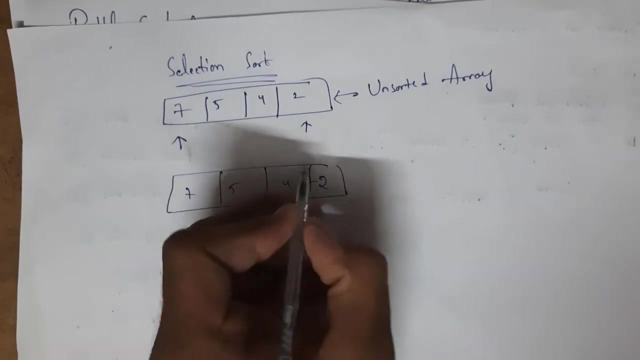 In an array and then it will place this minimum element at the beginning. So minimum element is 2.. So 7, 5, 4, 2 minimum element is 2.. So it will keep this 2 at the beginning and move this 7 in. 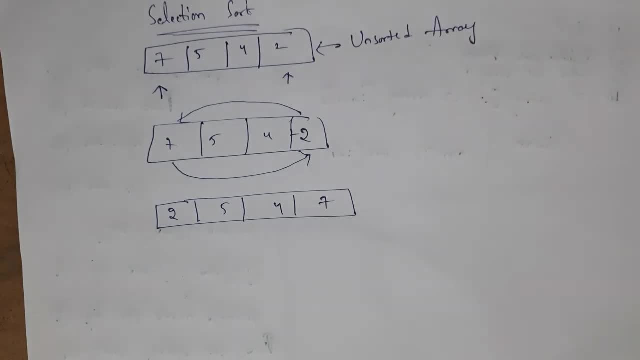 place of 2.. So 2, 5, 4, 7. Selection sort will find minimum element in an array and it will place this minimum element at the beginning. So, after placing minimum element at the beginning, it will consider this 2 as sorted array. So consider this 2 as sorted array, sorted, and consider this remaining. 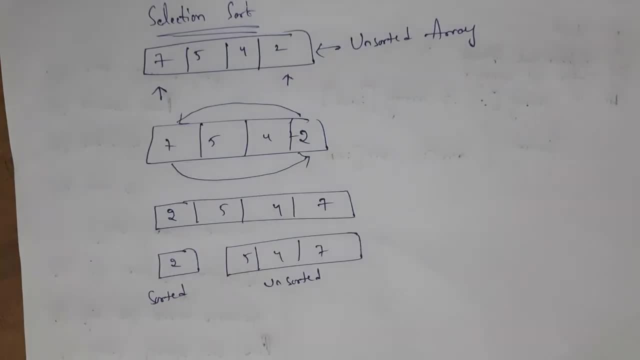 3 as unsorted array: 5, 4, 7.. Now again, we need to find minimum element from this unsorted array. Minimum element from this unsorted array is 4.. So we need to place this 4 at the beginning. So 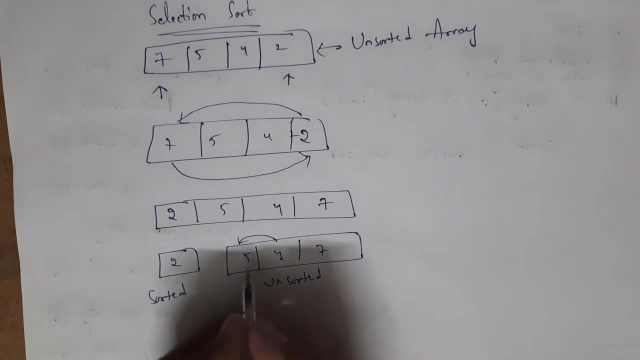 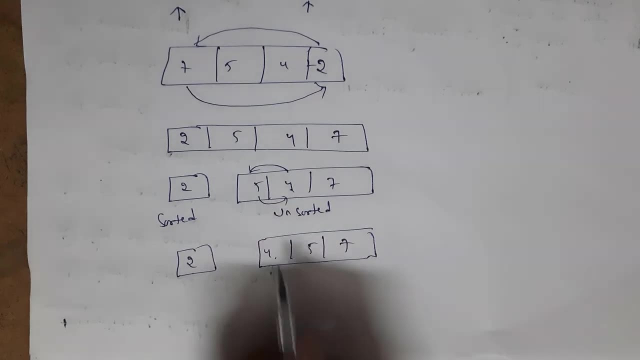 I mean, I am placing this 4 at the beginning and place this 5 in place of 4.. 2, 4, 5 and 7.. After placing minimum element at the beginning, consider this 4 as sorted array. So we need to write 2, 4. 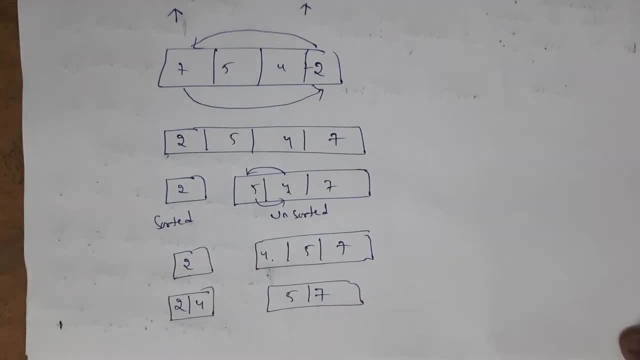 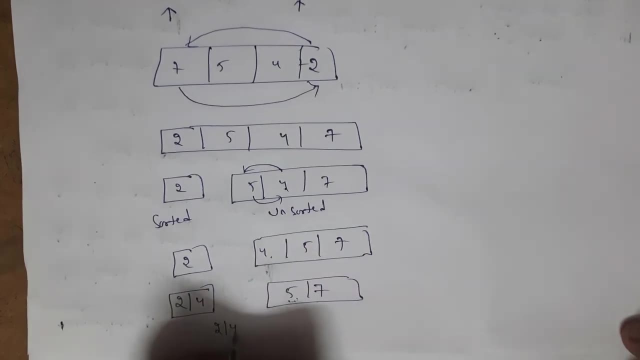 this is sorted array and this is unsorted array. now again, we need to find minimum element from this unsorted array. minimum element is 5. 5 is already at beginning, so consider it as sorted array. so 2, 4, 5 and it has 7. this is sorted array and this is unsorted array. this 7 is at the 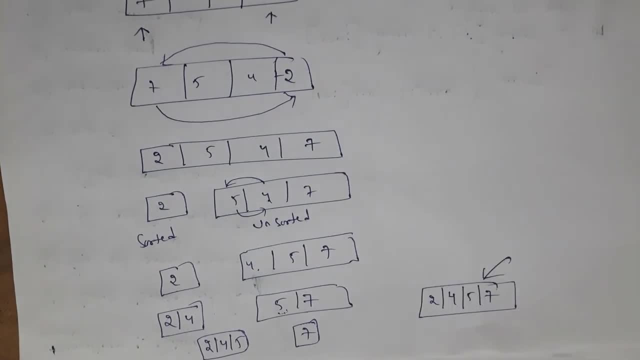 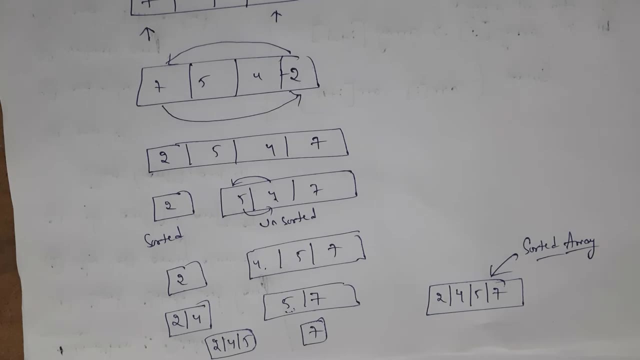 beginning. so again move this 7 into this sorted array. all these elements are from small to big, so this is sorted array. this is how we perform sorting by using selection sort. next i will explain algorithm for selection sort. here, step 1 is start and step 2 is selection sort of array. 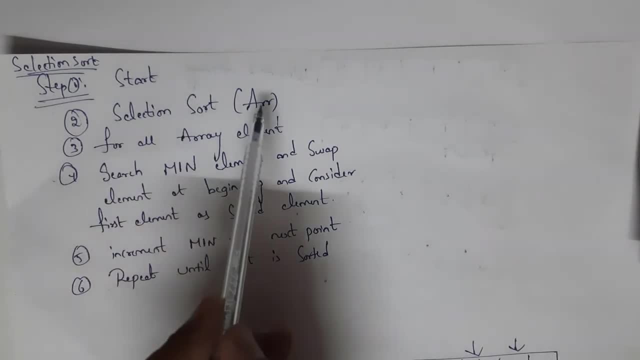 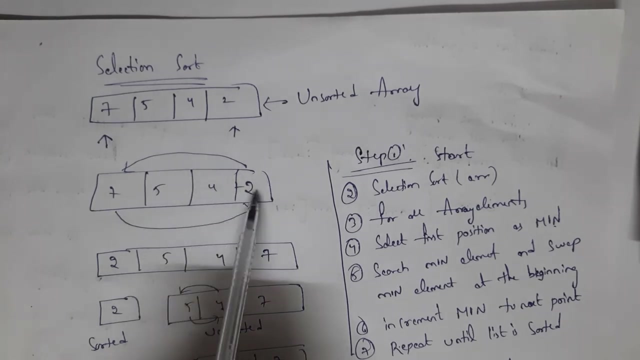 because we are sorting array of elements. so i written here selection sort of array and step 3 is, for all array elements, search minimum element and swap element at the beginning and consider it as sorted element, as i already explained in this before. example here smallest element is 2. 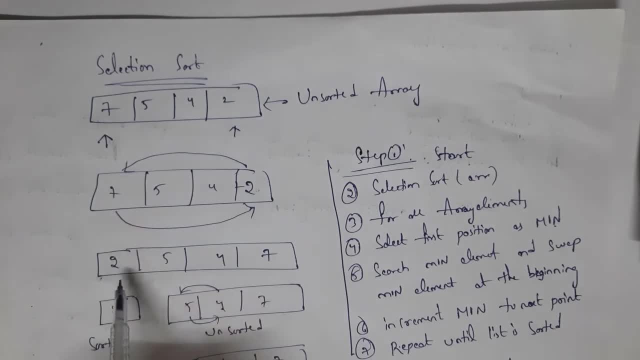 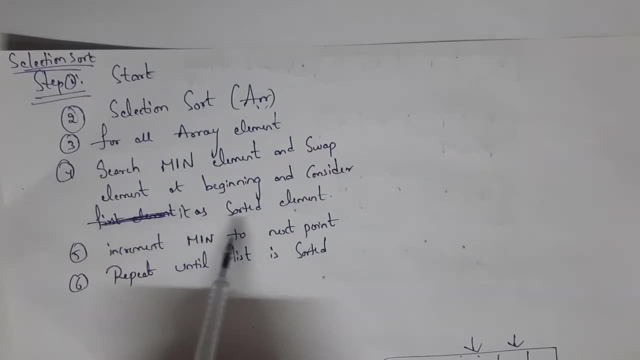 we will bring 2 at the beginning and then we will maintain this 2 as sorted array, and we need to maintain this process until complete list is sorted. so fifth step is increment minimum to next point and repeat until list is sorted. this is an algorithm for selection sort. this selection sort and bubble sort is not. 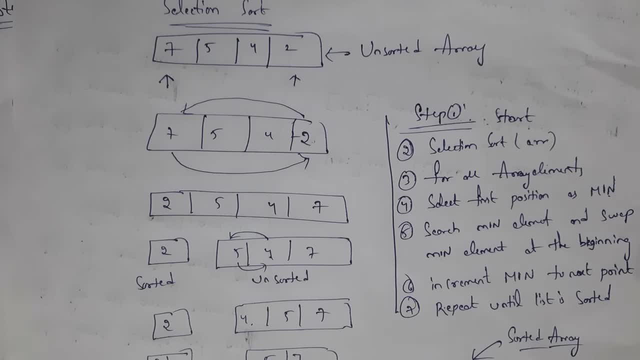 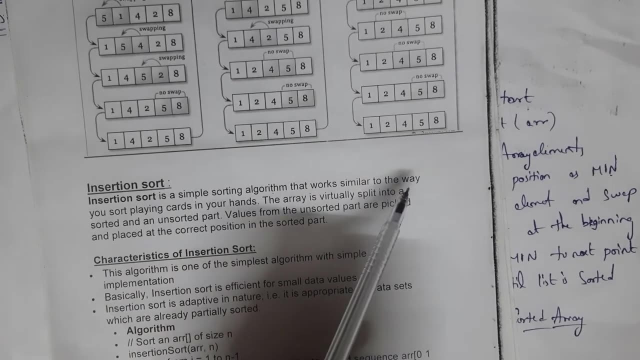 suitable for large size data sets. it is suitable only for small size data sets. next i will explain what is insertion sort. insertion sort is simple sorting algorithm that works similar to the way you sort playing cards in your hands. this insertion sort works same like how you sort playing cards in. 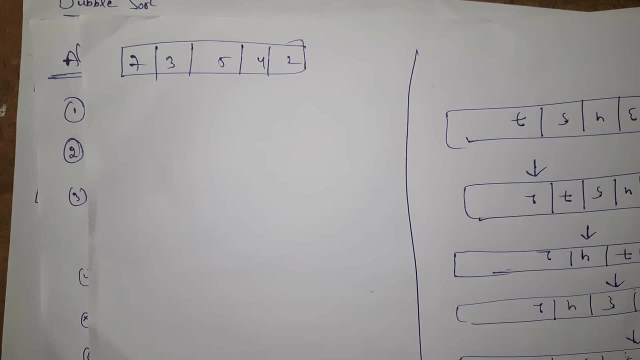 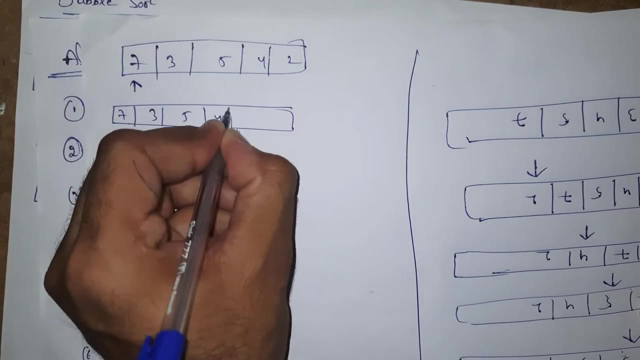 your hands. this is unsorted array. now we need to sort this array, and we need to sort this array by using insertion sort. at first, you need to place cursor at first position. after that, move cursor to next position: 7, 3, 5, 4, 2. move cursor to next position. this insertion sort works same like playing cards. 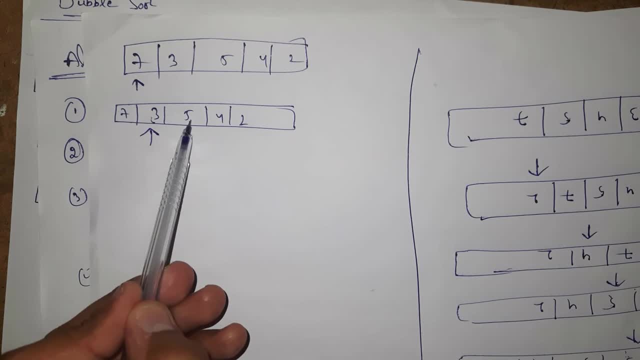 that means this 3 is compared with 7 and this 5 is compared with 3 and 7. 4 is compared with 5, 3, 7 and, at last, 2 is compared with all these remaining elements. based on this, you need to perform sorting. 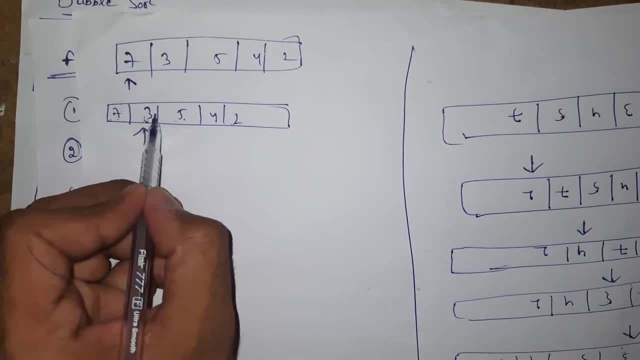 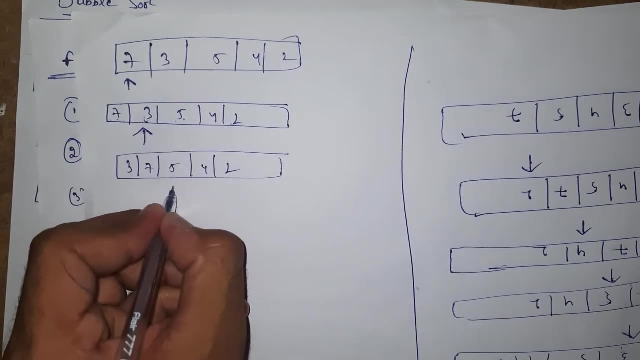 so whenever you move cursor to element 3, 3 must be here and 7 must be here. so you need to write like: 3, 7, 5, 4, 2, move, 3, move this cursor. next position, that is here. now again compare this 5 with remaining. 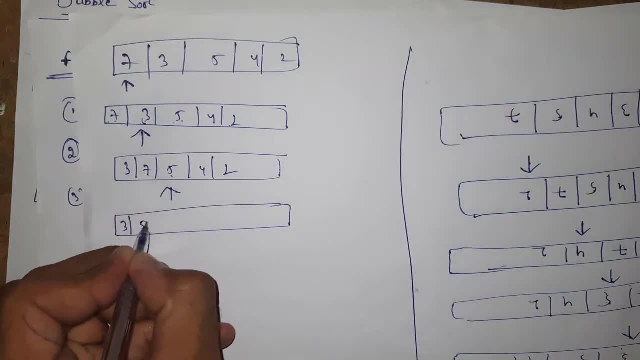 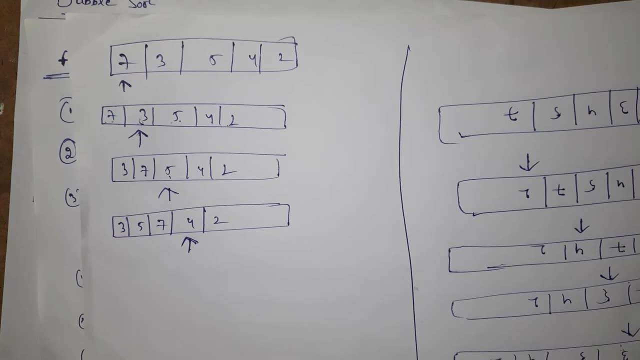 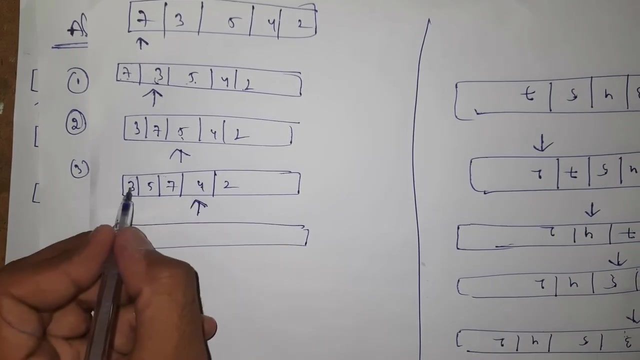 these two elements and arrange these elements in sorted manner: 3, 5, 7, 4, 2, 7, 4, 2. now again move cursor to one position forward, that is 4. place cursor at element 4. now compare this 4 with remaining elements, that is 3, 5, 7. actually 4 should be placed in between 3 and 5, so 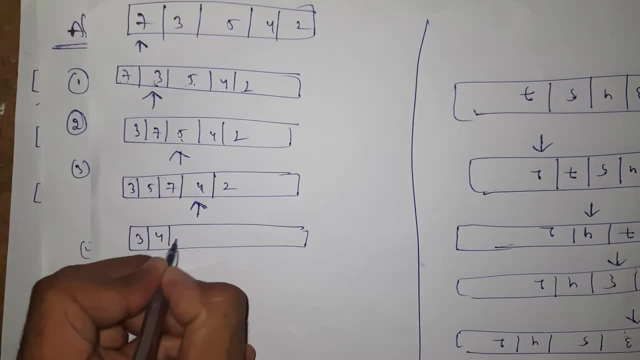 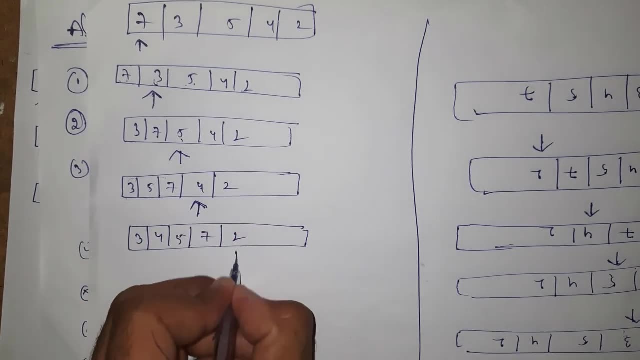 arrange this in sorted manner like 3, 4, 5, 7 and 2 at last move cursor. one position forward. that is, in place of 2, now 2 is compared with all these remaining elements, that is, 3, 4, 5, 7. actually, 2 must be its starting position. 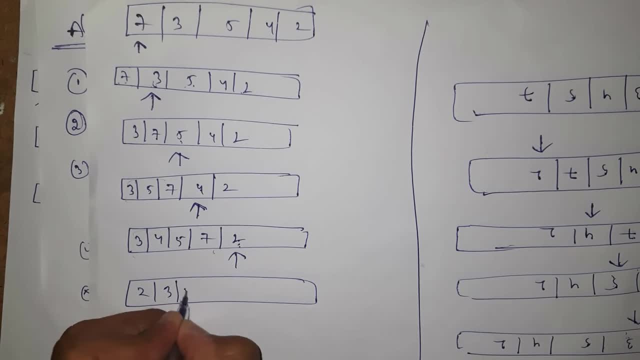 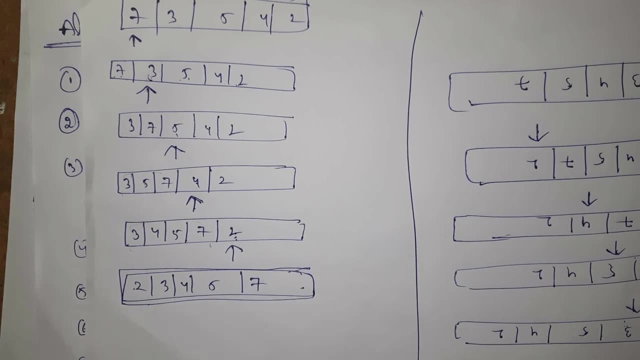 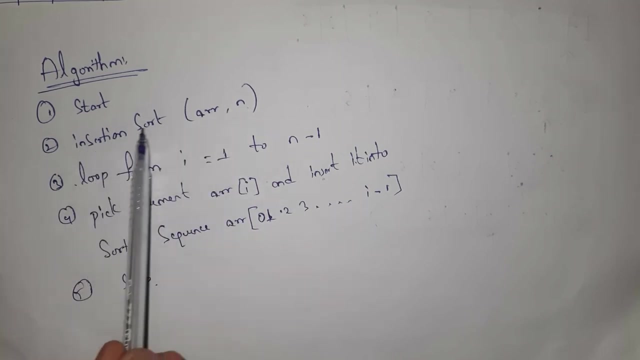 so arrange this in sorted manner like 2, 3, 4, 5, 7. now this is sorted array. now all these elements are from small topics. now i will explain algorithm for insertion sort. here step 1 is start and step 2 is insertion sort of array. comma n: that mean we are performing insertion sort on n number of. 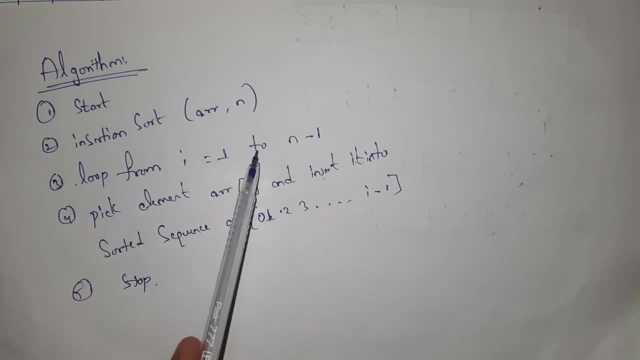 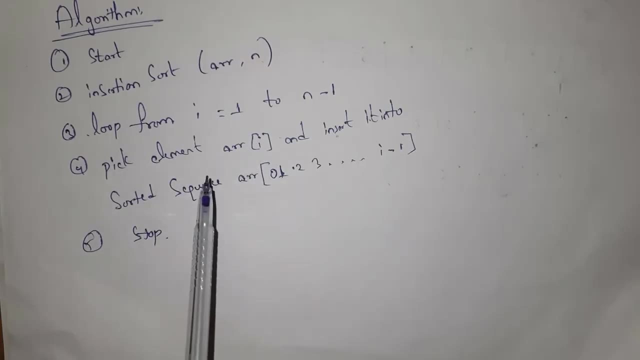 elements in an array and step 3 is from i equal to 1 to n minus 1, that is, from starting element to ending element. pick element. array of i. that mean we need to pick particular element and then we need to insert that element in sorted sequence that is like 1, 0, 1, 2, 3, so on i minus 1 and last. 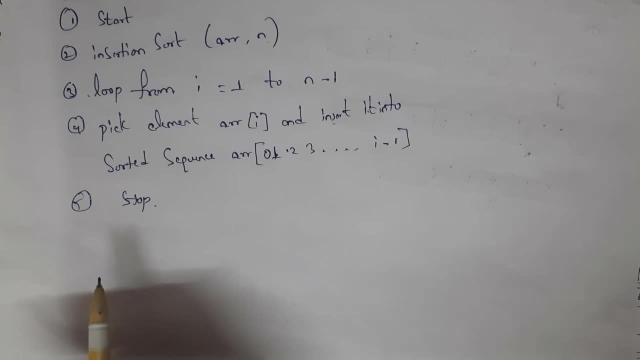 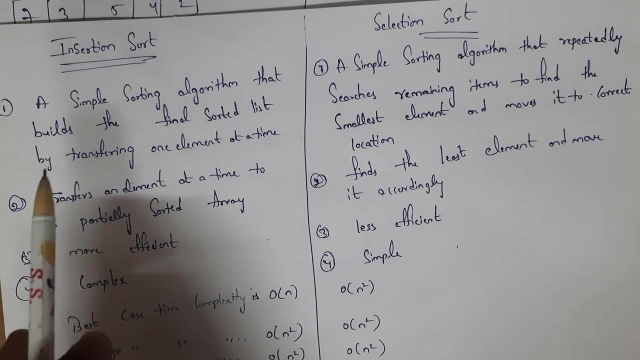 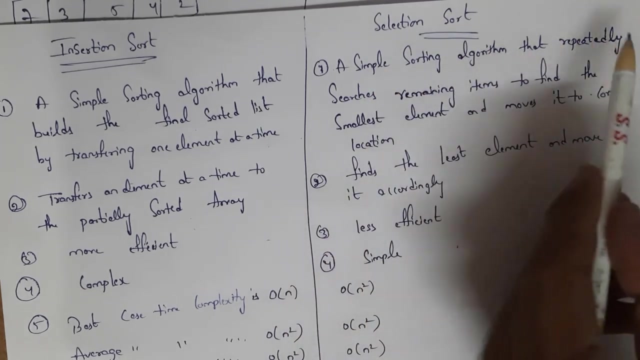 step is stop. next i will explain difference between insertion sort and selection sort. definition of insertion sort is a simple sorting algorithm that builds the final sorted list by transferring one element at a time, and this is definition of selection sort. selection sort is a simple sorting algorithm that repeatedly search remaining items to find smallest element and moves it to the 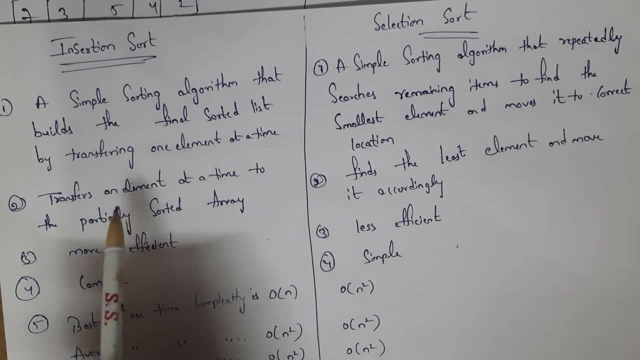 correct location. it transfers an element at a time to the partially sorted array and in selection sort it it finds least element and move it accordingly. insertion sort is more efficient when compared to selection sort and selection sort is less efficient when compared to. insertion sort is complex than selection sort and whereas selection sort is simple when compared to. 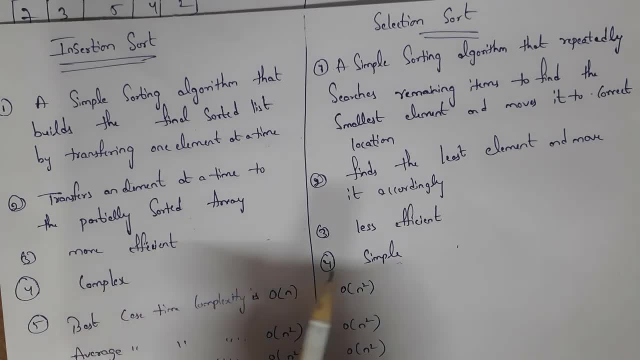 insertion sort. insertion sort is more complex than selection sort, and whereas selection sort is very simple, when compared to insertion sort, best case time complexity of insertion sort is big o of n and average and worst case time complexity of insertion sort is big o of n square, and, whereas 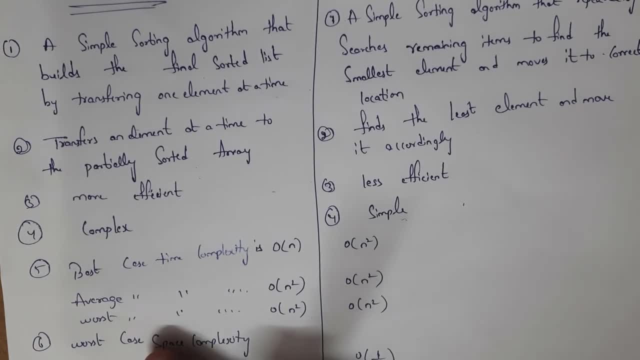 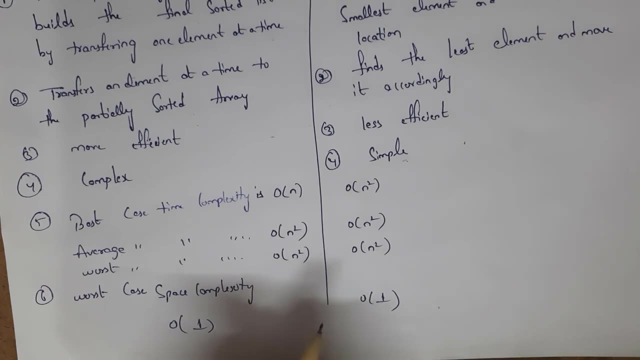 best case, average case and worst case time. complexity of selection sort is big o of n square. worst case space. complexity of insertion sort is big o of one, and whereas worst case space complexity of selection sort is big o of one.